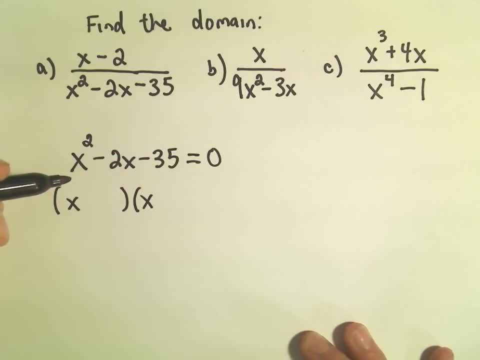 I think we can factor that. So I need two numbers that multiply to negative 35, but add up to negative 2. So I think some combination of 7 and 5 will work. Since the middle term is negative, that means the bigger of these two numbers gets the negative sign. 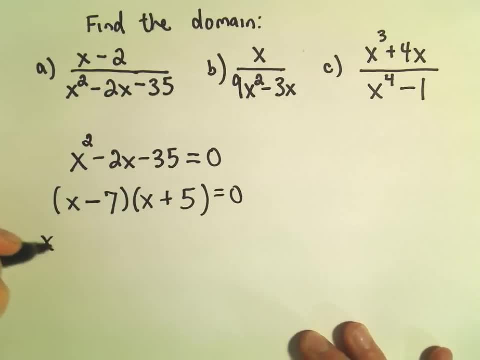 So, all right, I think that looks like a correct factorization. And now we simply set each factor equal to zero and solve. So for the first part, if we add 7,, we would get x squared, So we get x equals 7.. And if we subtract 5,, we would get x equals negative 5.. 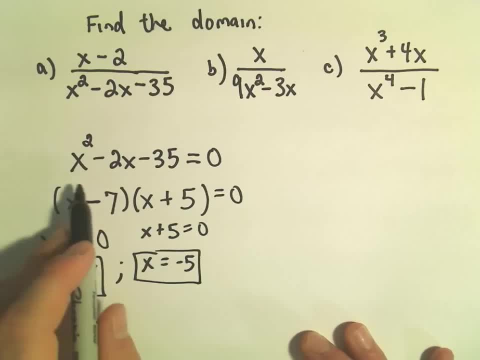 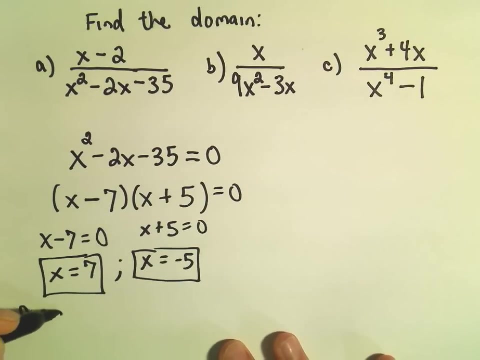 So those are the solutions to the equation. x squared minus 2x minus 35 equals zero. So again, what that says is it says 7 and negative 5 will produce zero in the denominator and that's bad. So in this case we would say the domain is all real numbers. 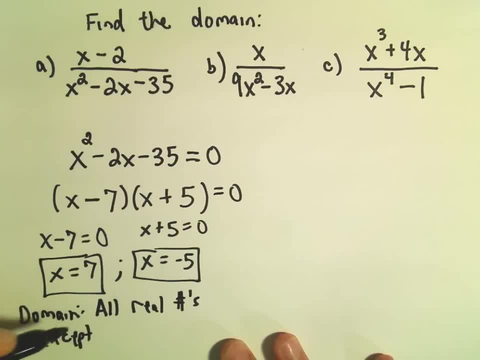 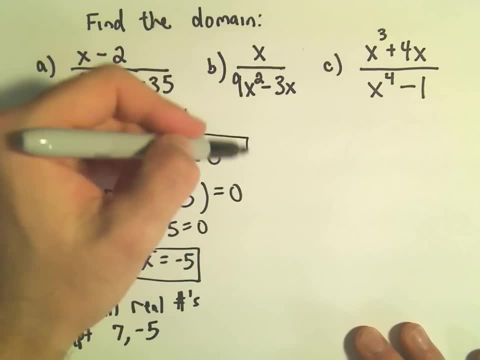 So all real numbers. So all real numbers, All real numbers, except 7 and negative 5.. Okay, so that's it. That's the main idea. So let's do these other two examples real quick. So part b: we have x over 9x squared, minus 3x. 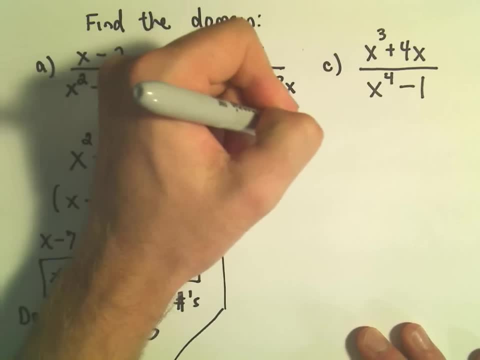 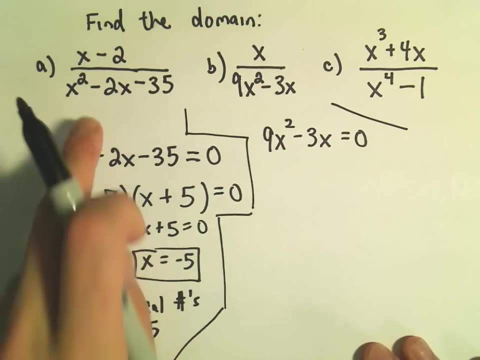 Again, I'm just going to take the denominator 9x squared minus 3x, and I'm going to set that equal to zero. Okay, so again you know, I've got notice. they're all quadratics, or, excuse me, the first two are quadratics. 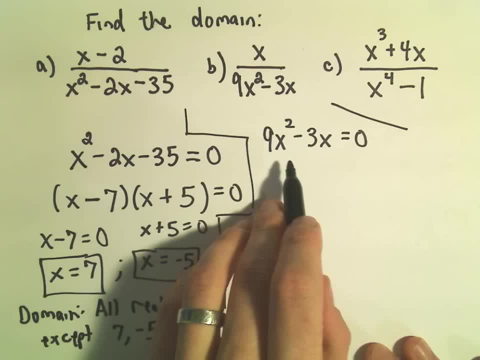 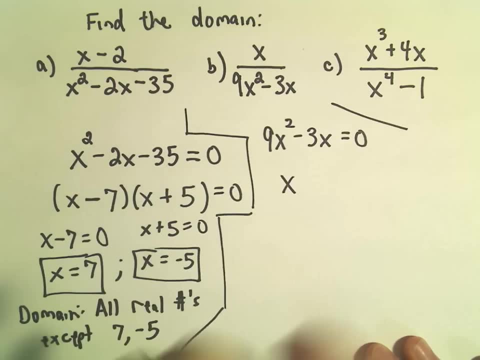 The last one is not. It's not quite quadratic, but it'll still factor. So for this quadratic I notice there's no constant, so I can certainly factor out an x, And also there's a 9 and a 3.. 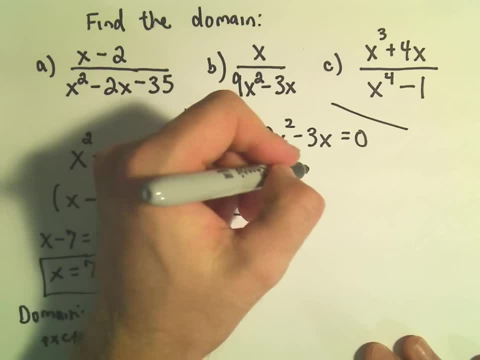 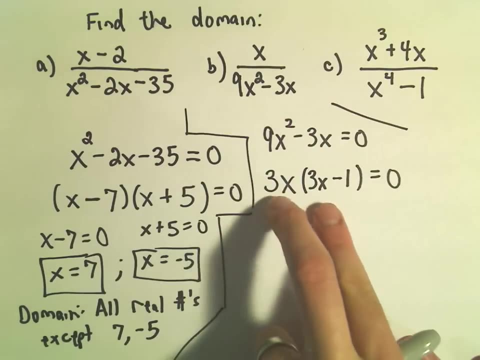 Well, I could factor out the greatest common factor, which is 3. And then, I guess in parentheses, I would need a 3x back and then a negative 1.. So if we multiply that out, we would get 9x squared minus 3x. 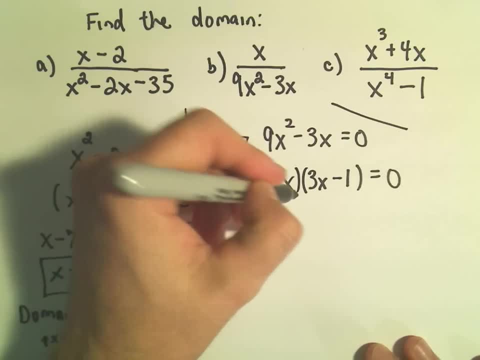 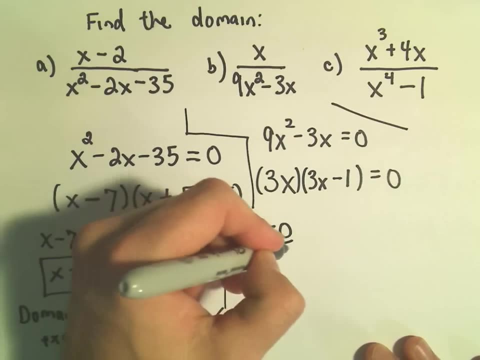 And again, we just set each part equal to zero, each factor. So if we set 3x, we would get 9x squared minus 3x. So if we set x equal to zero, if we just simply divide both sides by 3, we would get x equals zero. 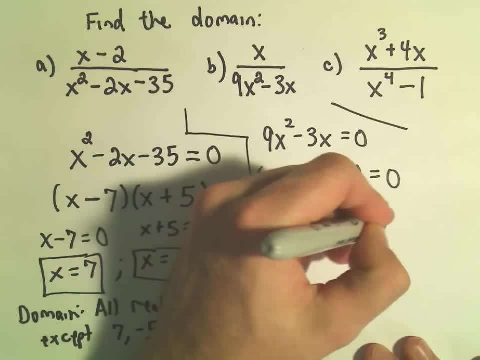 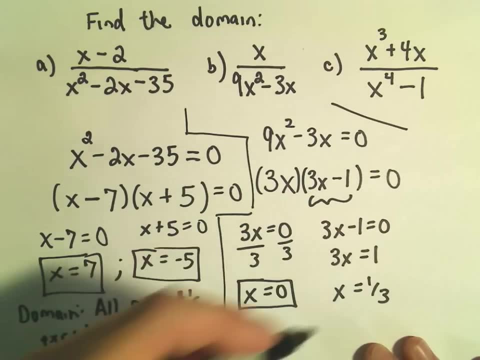 And if we set the 3x minus 1 equal to zero, well, I could add 1 to both sides And then we could divide by 3. We would get x equals one-third. So again, what I'm finding is I'm finding the values of x that have to be excluded. 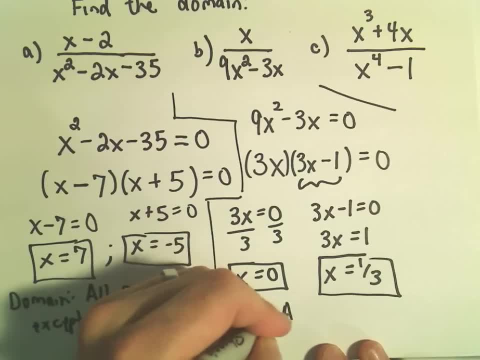 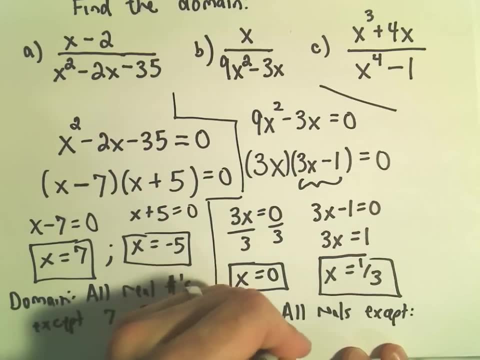 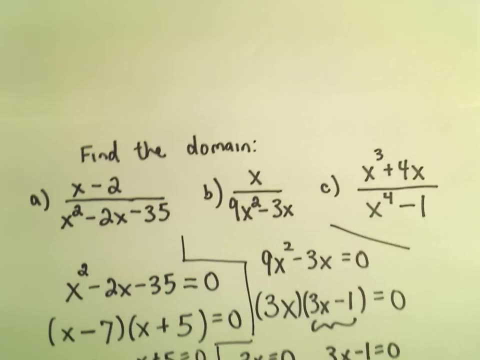 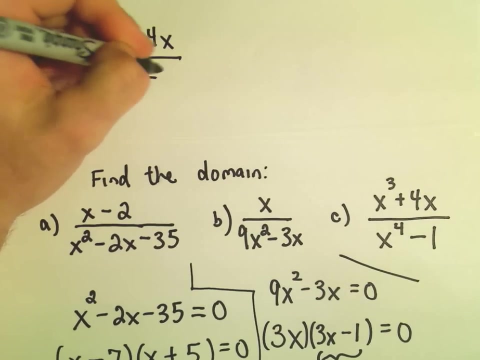 So again, the domain would be all reals, Except That x equals zero and x equals one-third. So let's do our last example here. Let me copy it down, since I ran out of room. So x cubed plus 4x over x to the fourth minus 1.. 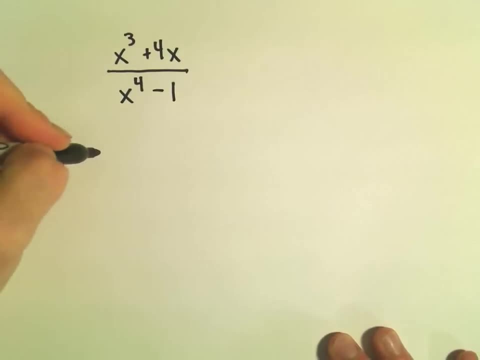 So same thing, Let's just find the domain of it. So I'm going to set the denominator x to the fourth minus 1, equal to zero, And in this case I believe we could factor this actually to get the x to the fourth. 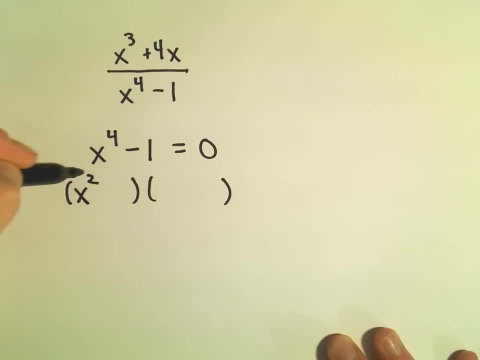 So this is a difference of perfect squares. So to get the x to the fourth, we could use x squared and x squared, And then to get the negative 1, we could simply use negative 1 and positive 1.. OK, So now I'm going to ask myself, you know, can I factor this any further? 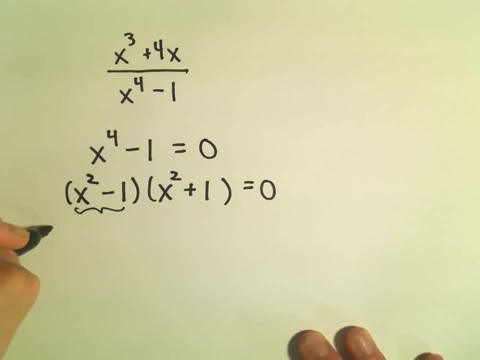 Well, x squared minus 1 is again a perfect square. We can factor x squared minus 1.. As x minus 1, x plus 1.. And then I have to ask myself: you know, does x squared plus 1,, does that factor? 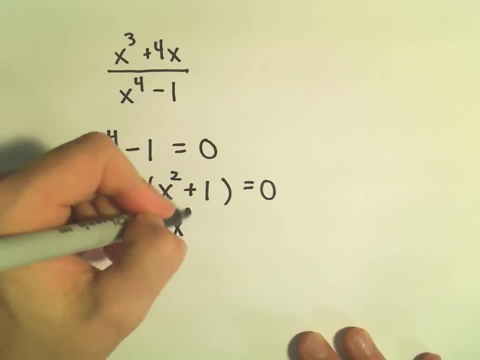 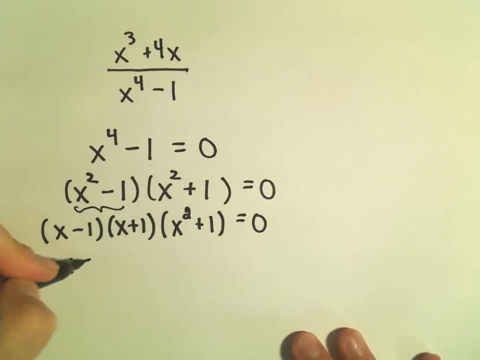 And you know you can play with it, But it turns out for sure that it does not factor. So I'll just drop that right down. And again now, I set each part equal to zero, each factor. So I set x minus 1 equal to zero. 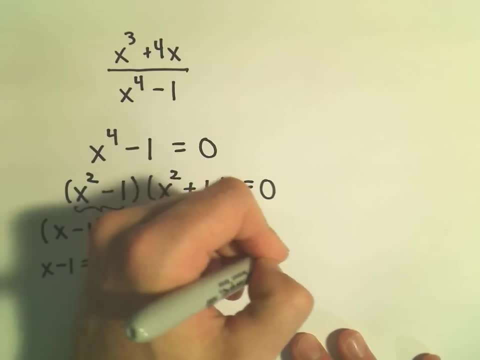 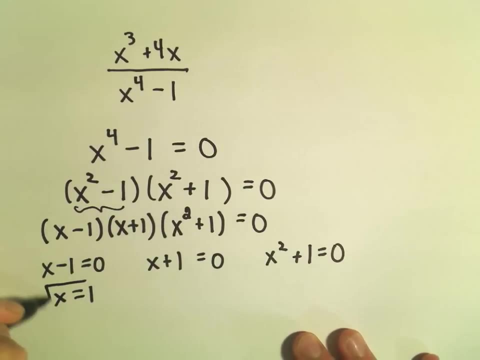 I'm going to set x plus 1 equal to zero. I'm going to set x squared plus 1 equal to zero. So for the first part, I'll just add 1 and get x equals 1.. So that's going to be a value that has to be excluded from the domain. 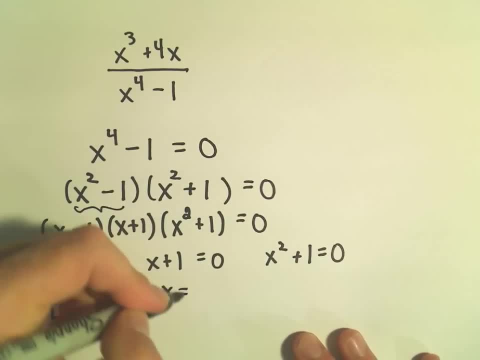 From our middle equation. we could simply subtract 1 and get x equals negative 1.. So that'll be a value that has to be excluded from the domain. You can almost reason out. Well, you can probably reason out that this last equation doesn't have solutions. 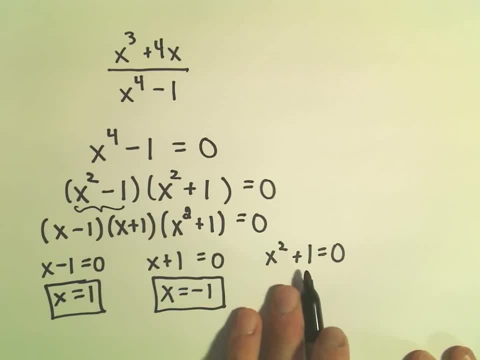 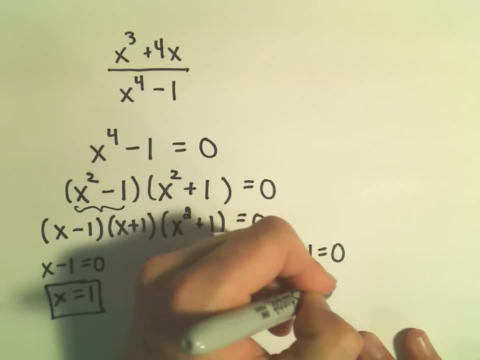 I mean, what numbers can you square and add 1 to them and get 0 out? So maybe think about that, But maybe you try to figure it out, Maybe you try to factor it, or maybe you tried to solve it by subtracting 1 and then you tried to take the square root of both sides.